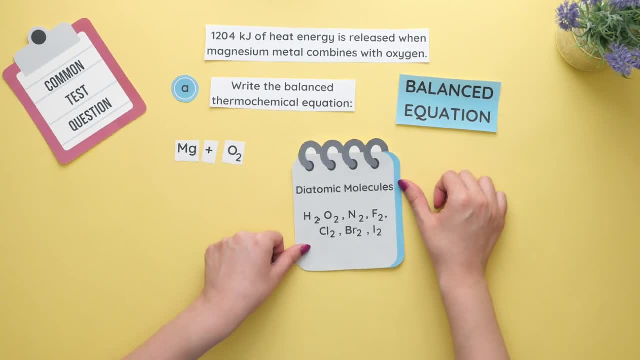 oxygen is a type of diatomic molecule. Diatomic molecules are atoms that exist in pairs. When we combine magnesium and oxygen together, we are only looking at one oxygen, so ignore the subscript of two and we will identify our charges. Magnesium has a plus two charge and 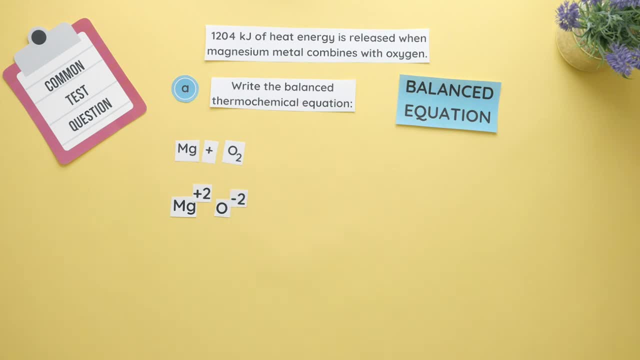 oxygen has a negative two charge. Since the charges are the same number and opposite signs, we do not need any subscripts. so our product is magnesium oxide. Balance the chemical equation by separating each element and counting how much of each element there is on either side. On the reactant side we have one. 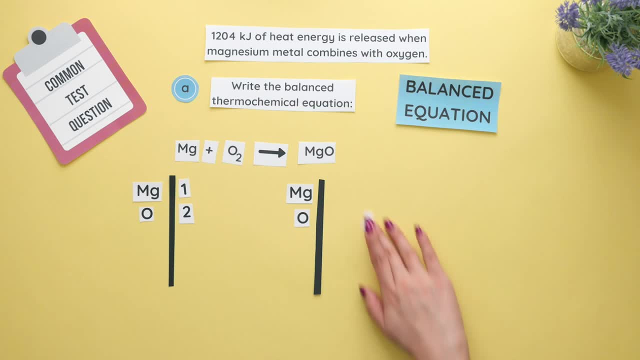 magnesium and two oxygens and on the product side we have one magnesium and one oxygen. We need to balance out the oxygens, so we'll add a two in front of our product and we now have two magnesiums and two oxygens on the product side. So now the magnesium needs a two in front on the reactant side and 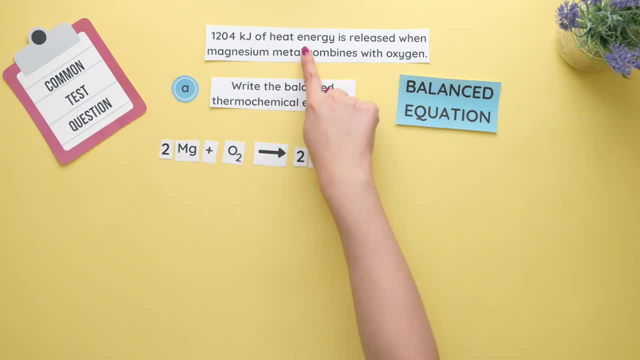 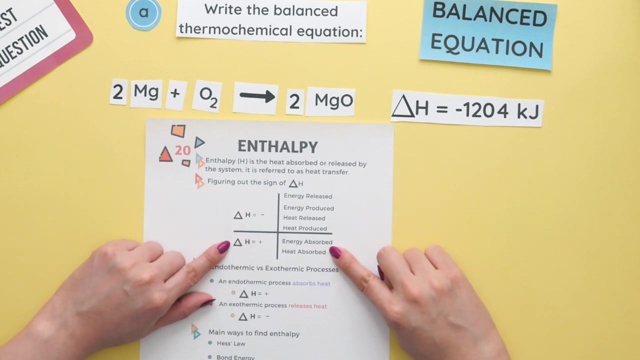 this is our balanced equation. This question also states heat energy is released, meaning our enthalpy change is released, which means it's negative. Note: if heat or energy is released, then our enthalpy change is negative. If heat or energy is absorbed, then our enthalpy change is positive. We'll use 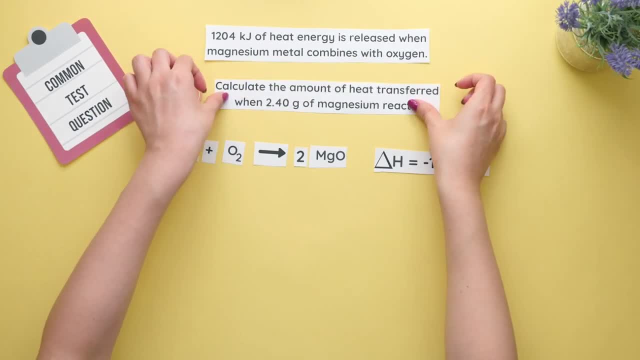 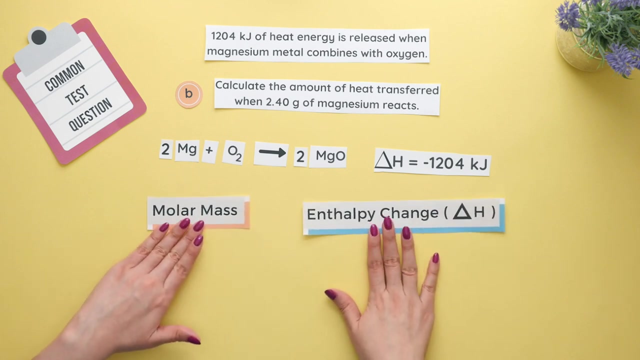 everything we found in part A for part B, which states: calculate the amount of heat transferred when 2.40 grams of magnesium reacts. So we're given the mass of magnesium and we're finding heat. We'll use the main conversion factors we discussed at the beginning of this video, which were molar mass and enthalpy. 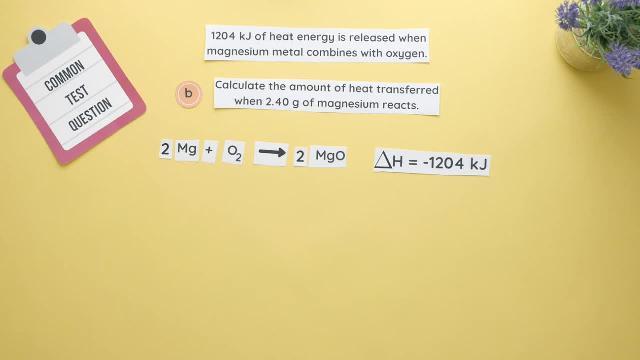 change To get from grams to kilojoules, which is what heat is measured in, we will go from at the grams of magnesium to the moles of magnesium to kilojoules. Always start with what we are given, which was the 2.40 grams of magnesium. To convert grams to moles, we will use the 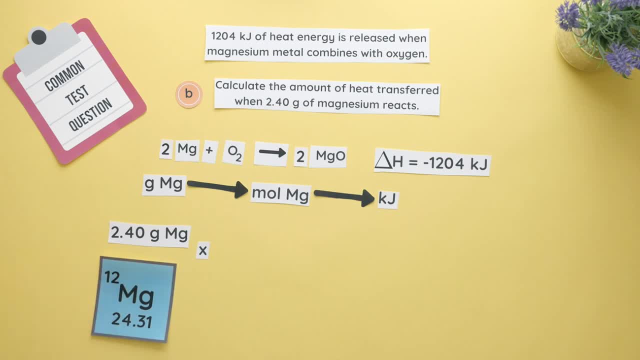 molar mass of magnesium, which is found on the periodic table, Allign grams across from each other, so they can cancel. and now we are at moles of magnesium. Next, we need to convert to kilojoules using the given enthalpy change found in part A, Our units for enthalpy change. 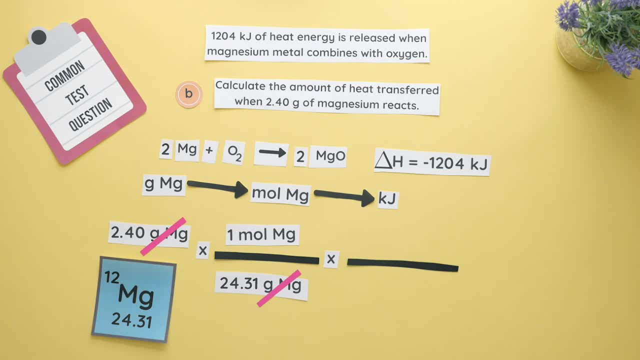 are really joules per mole. So, since we are looking at magnesium, our conversion factor will include the number of moles we have for magnesium in our balanced equation, which is 2.. We'll place 2 moles of magnesium on the bottom, since we want to align our 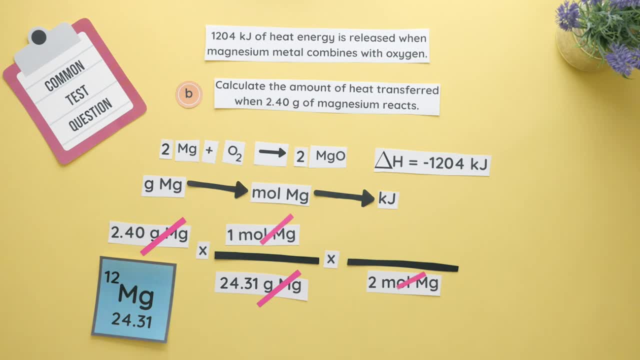 units of moles to cancel out, and on top we will have our kilojoules, since this is what we're looking for. Multiply each number straight across, then divide by the numbers multiplied and round to 3 sig figs, since our given value had 3. 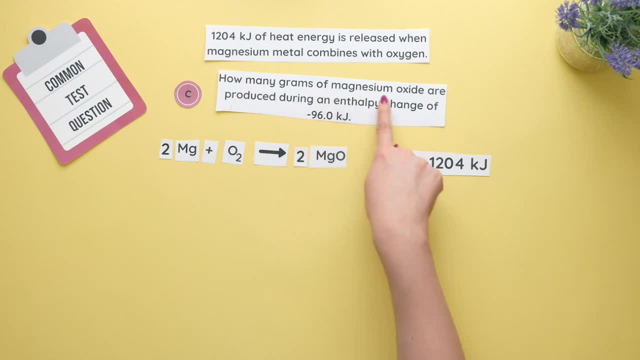 sig figs, Part C states how many grams of magnesium oxide are produced during an enthalpy change of negative ninety six point zero kilojoules. So we are given our enthalpy change of negative ninety six point zero kilojoules and 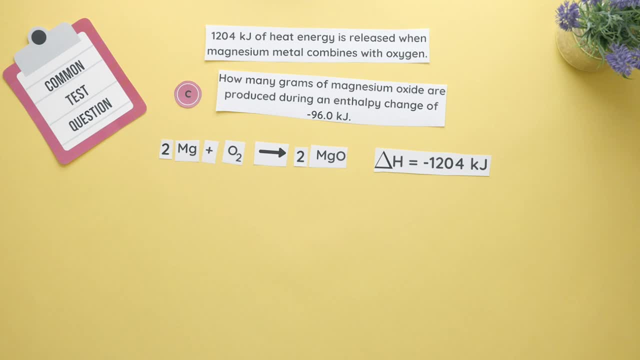 asked to find the grams of magnesium oxide. We'll start with the given unit of kilojoules and make our way to moles of magnesium oxide. then, using the molar mass of magnesium oxide, we'll find the grams. Our setup will start with our. 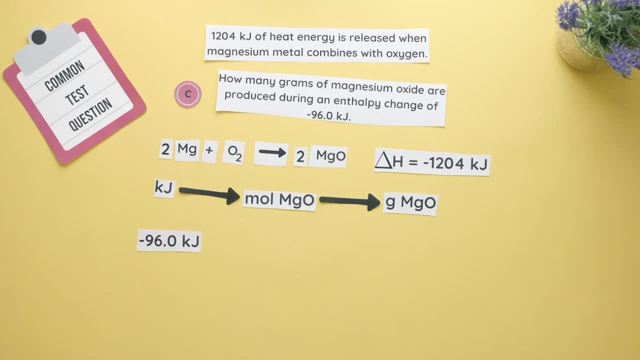 given value of negative 96.0 kilojoules and we will use the enthalpy change as our conversion factor. This time it's flipped because we always align our units so they can cancel out. So kilojoules goes on the bottom. 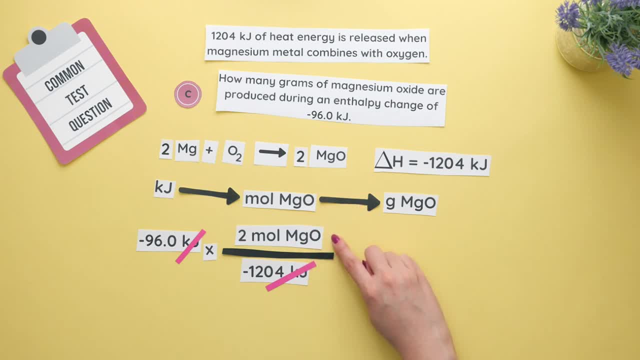 and two moles of magnesium oxide goes on top. We found this from our balanced equation. Next, we will convert our moles of magnesium oxide to grams, so we'll use the molar mass of magnesium oxide. To find the molar mass of magnesium oxide, we will add up each element's individual mass and 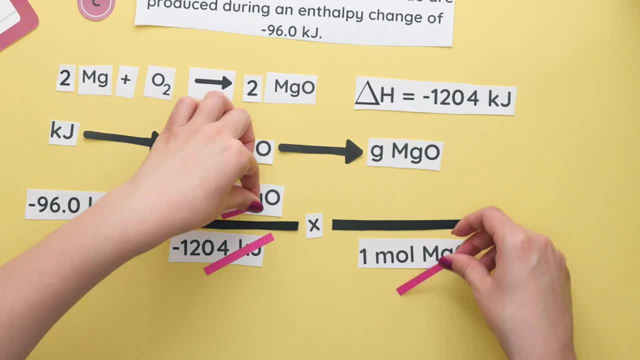 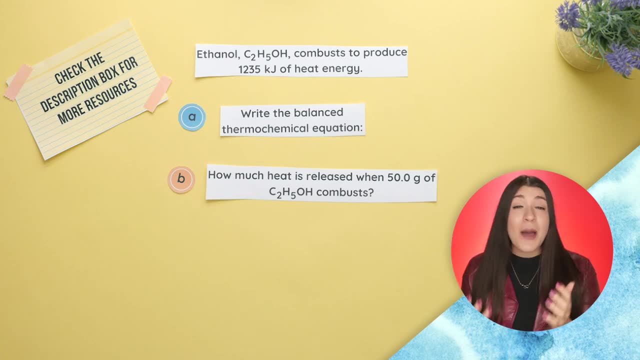 get 40.31 grams per mole. The moles cancel and we get 6.43 grams of magnesium oxide. Try this question out on your own and we'll go over the step-by-step answers in this next video. And if you'd like more chemistry, help make sure to check the description box for my recommended resources.